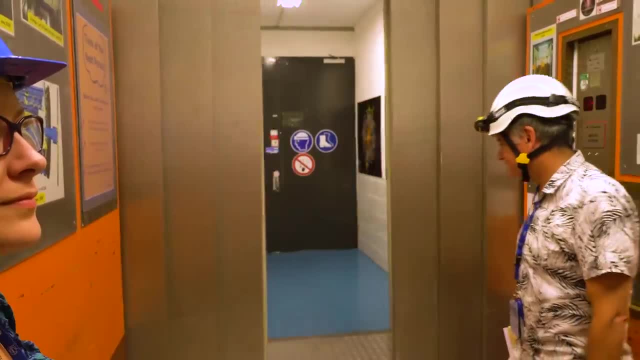 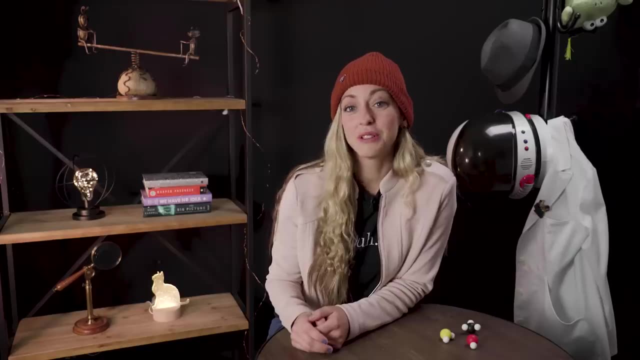 You descend 100 meters in an elevator, You get briefed on not using the stairs if anything goes wrong And you stop to admire the strange signs and equipment. And if you devote two entire days of your life, you might just get to see a couple of. 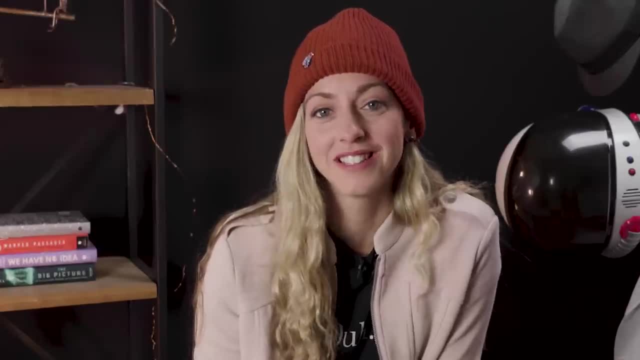 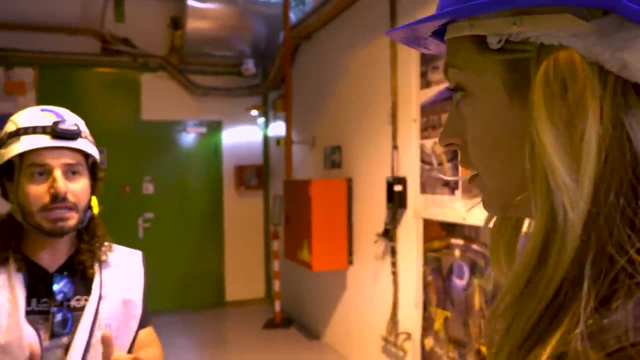 the detectors Like we did. We were there for a while. I think they wanted us to leave. We're about to go down in CMS, So the elevator is like the safest place to be. Yeah, So if there's any emergency, that's the sort of meeting point. 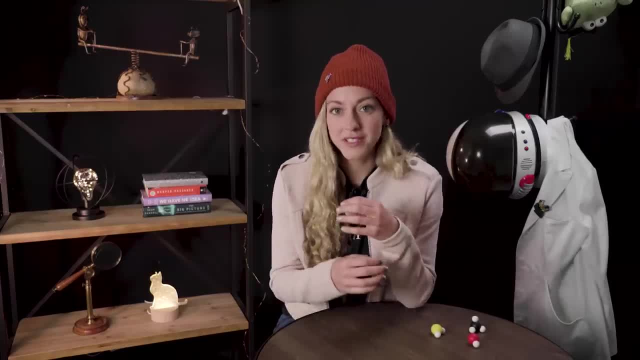 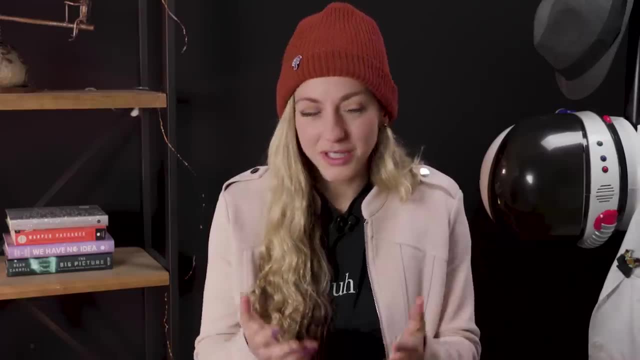 This is the video where I get into the elevator. This is the essence of CERN: It's the most advanced and expensive scientific lab on Earth And it's used to study particles- I know not the most fashionable area of physics upon first inspection. 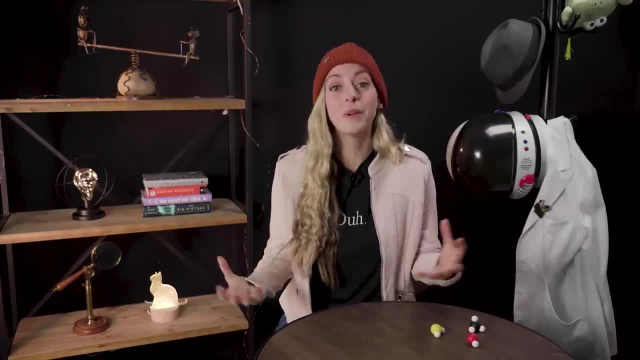 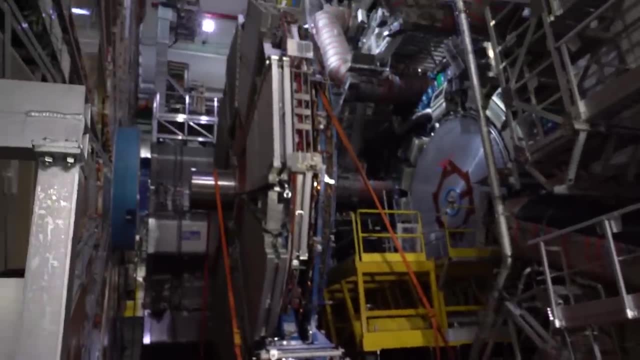 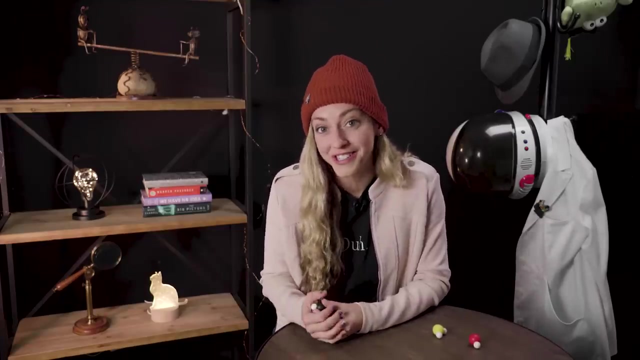 But it's the most fundamental question. It's the one we all asked when we were kids: What are we all made up of? What are the fundamental particles that make up everything in the universe? Oh sorry, And how did these detectors go about answering that question? 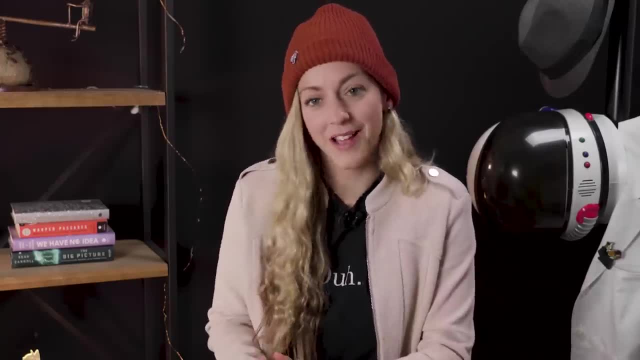 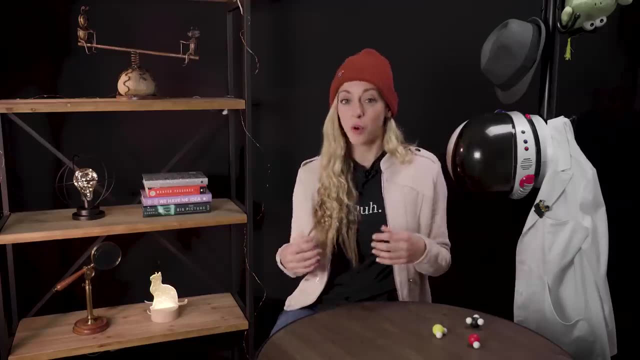 This is what I was most interested in, And it was a bit of a rough start because after three minutes of thinking I realized I didn't even know what a particle is. Turns out that I don't know what a particle is because I never got to quantum field theory. 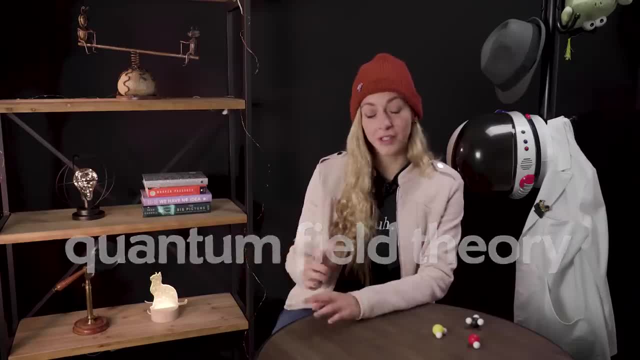 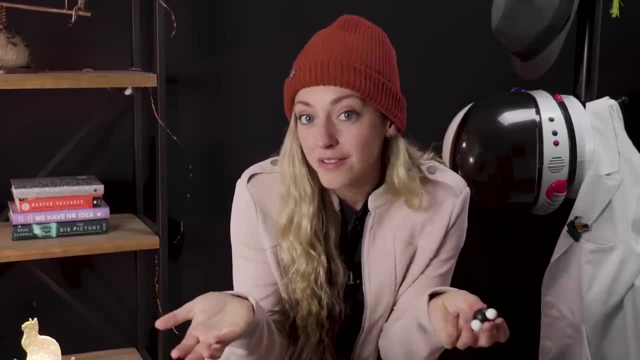 in my physics classes. So if you don't know either, join the club. So let's start there. What are these particles that CMS is studying Like, say, the Higgs boson? The Higgs was discovered in 2012.. 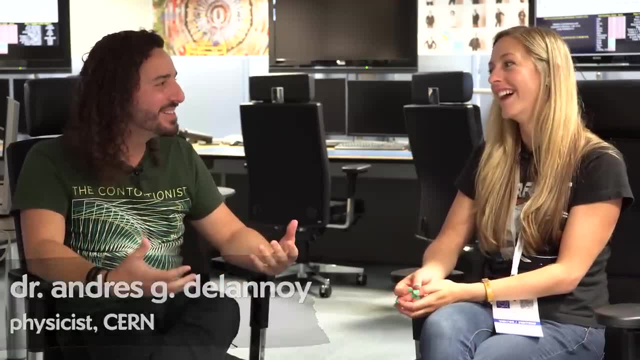 2012.. July 4th, So we call this Higgs Dependence Day. The discovery of Higgs was discovered in 2012.. 2012.. The discovery of the Higgs was the crowning achievement of the Large Hadron Collider at 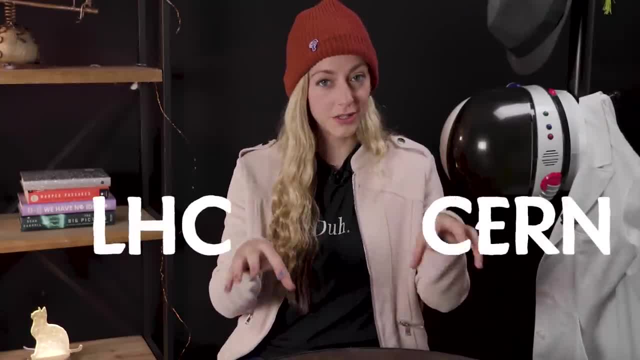 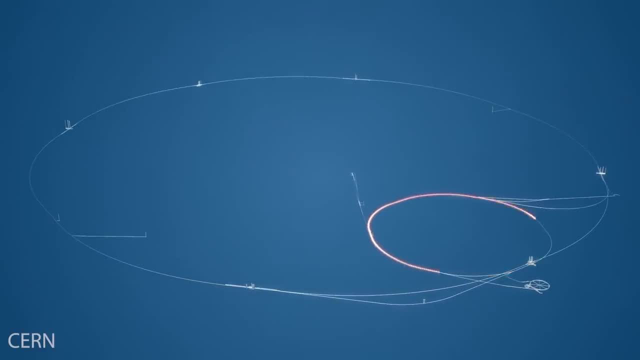 CERN. By the way, the Large Hadron Collider, the LHC, and CERN are two different things, which I didn't really know going into my tour at CERN. The Large Hadron Collider is the giant ring, the particle collider, that is part of the. 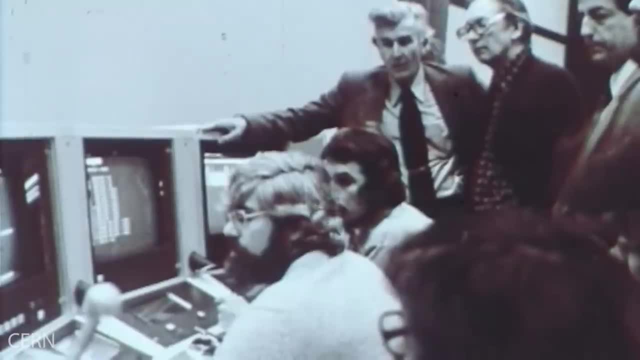 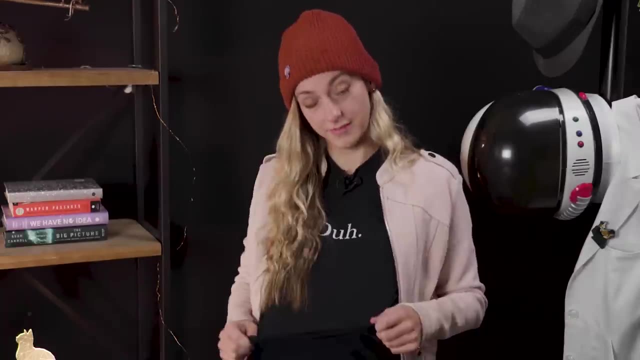 facility, the entire place called CERN. There are actually smaller colliders that were built starting in the 50s. I didn't know any of this, But the Large Hadron Collider is the large ring that collides hadrons, Duh. 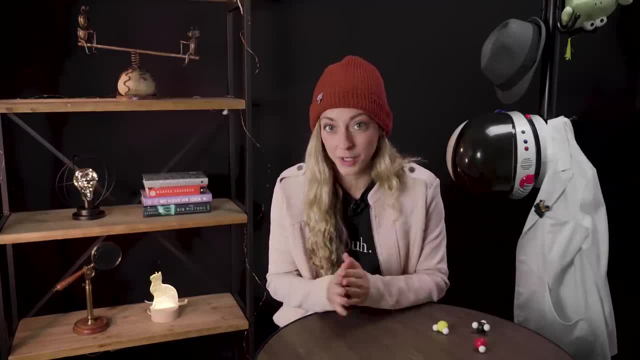 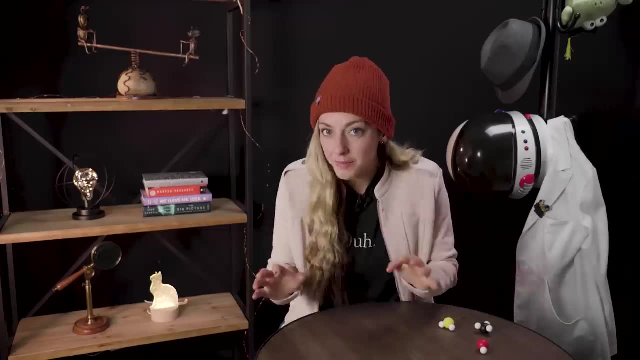 Anyways, the discovery of the Higgs. The Higgs is the tip of the iceberg when it comes to particles. It's just one of 30 fundamental particles that make up everything in the universe. Take any material, any wood, any frogs, any cats, any aliens, any snatoms, shout out to. 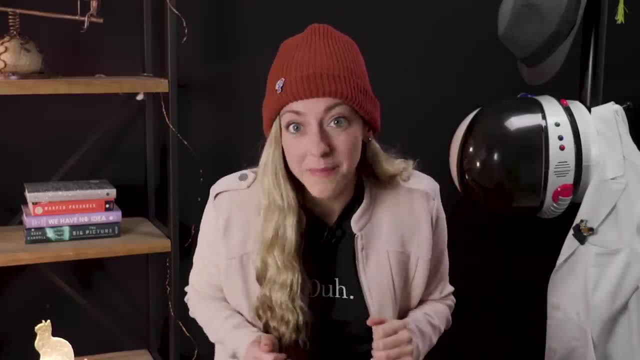 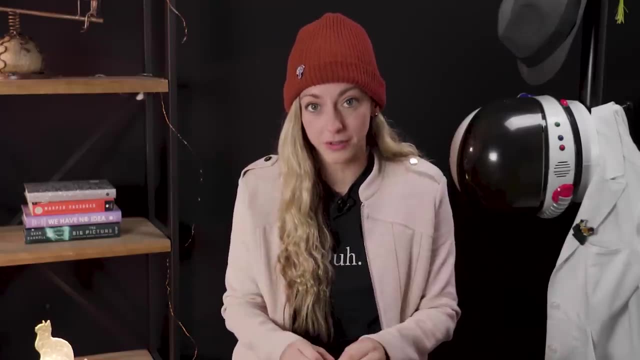 Derek any derricks, any non-materials like antimatter or even beams of light, break them down into their fundamental bits and you'll get 30 fundamental particles, Maybe 31 if you count the graviton, but let's not. 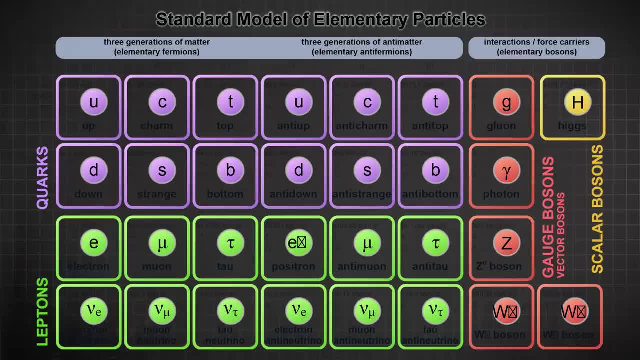 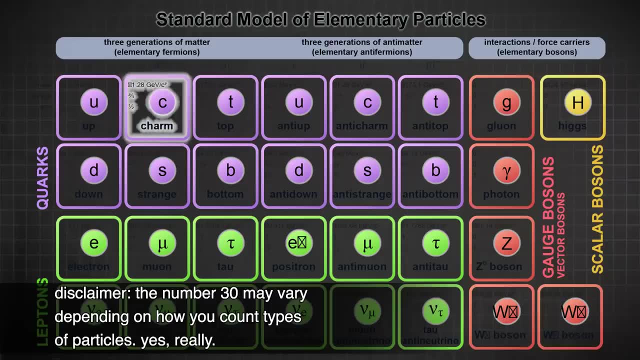 Because it's not a big deal. It's not observed. So 30 fundamental particles in the standard model of particle physics. I'm not going to read off all the particles because there are too many, but there are some fun ones to say, like the charm quark and the gluon, and some familiar ones like 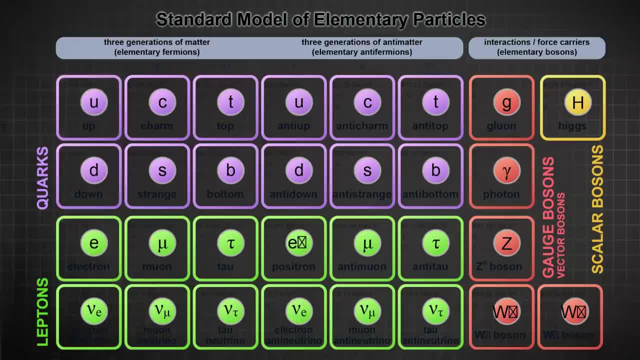 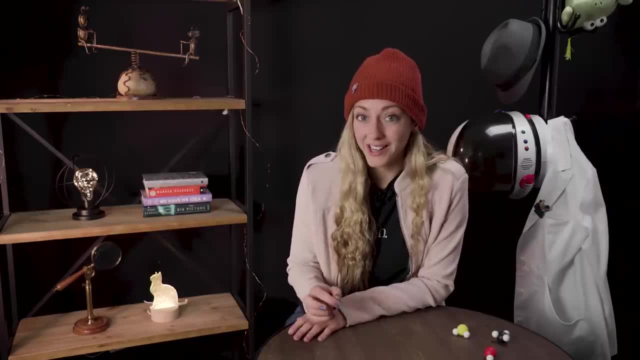 the electron, the photon and the up and down quarks. Okay, maybe those are not as familiar, but those are the ones that make up neutrons and protons. So elegant, But the real story is more complicated. The universe is actually made of quantum fields, not particles, if you want to be really accurate. 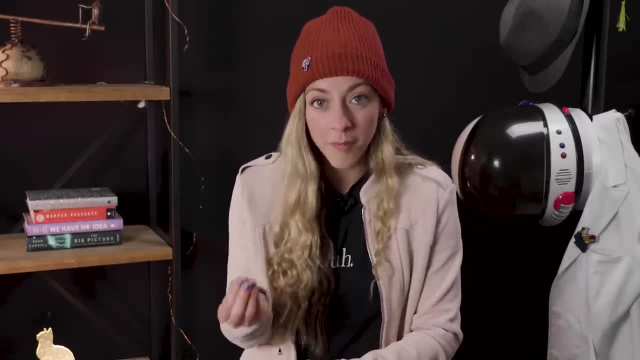 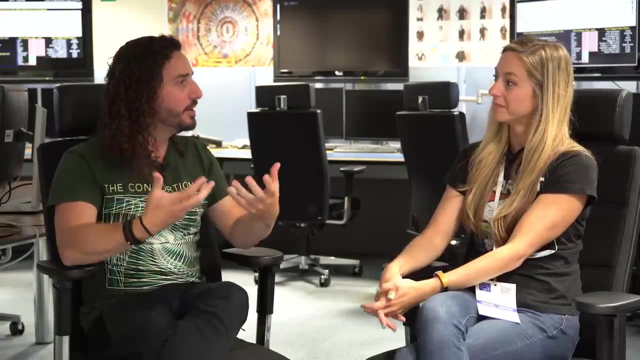 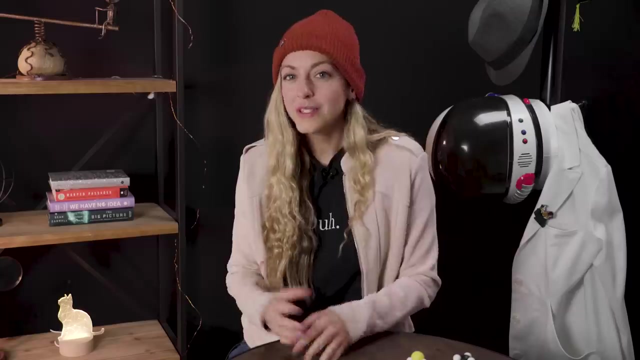 And if you want to know what particles are, Because particles are a phenomenon that emerges from quantum fields. The universe is a collection of these quantum fields. For each particle, there's an associated quantum field. Of course, for the photon, the associated quantum field is the electromagnetic field. 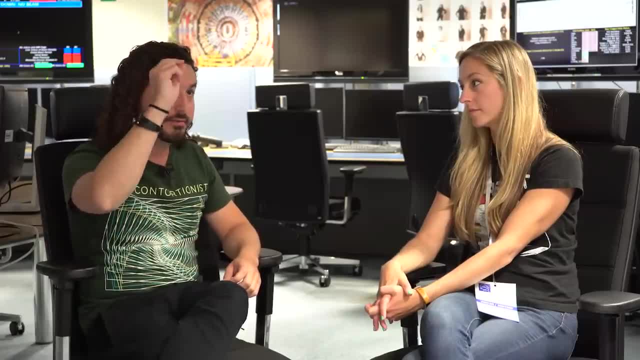 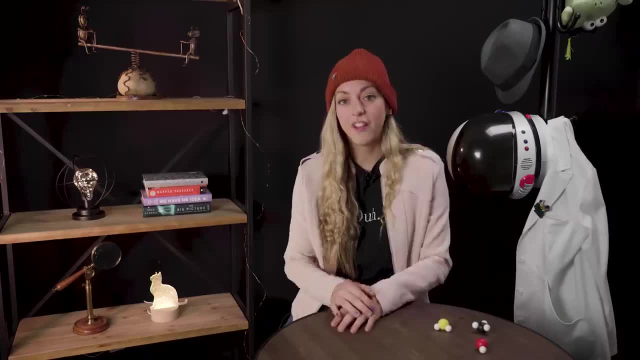 What's a field? What I mean by a field is just having a value, a number perhaps, at each point in space that can evolve with time. A field is like a grid, Like a grid, Like a 3D map onto all of space. 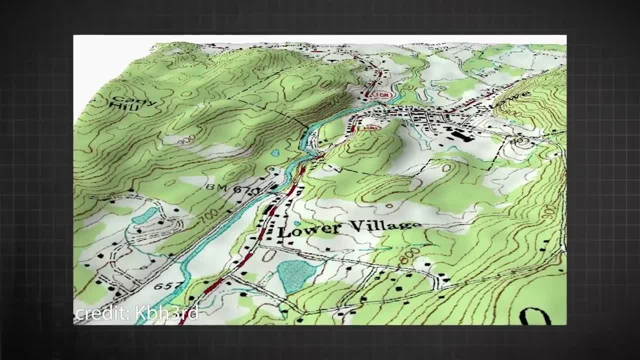 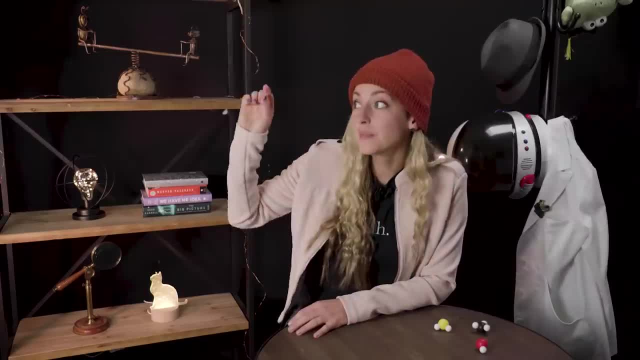 It's like a topographical map with numbers, Except instead of showing hills and ditches, with a quantum field, you measure something like the energy density of the gluon field. Even if this point in space right here doesn't have an electron, it still has a value for. 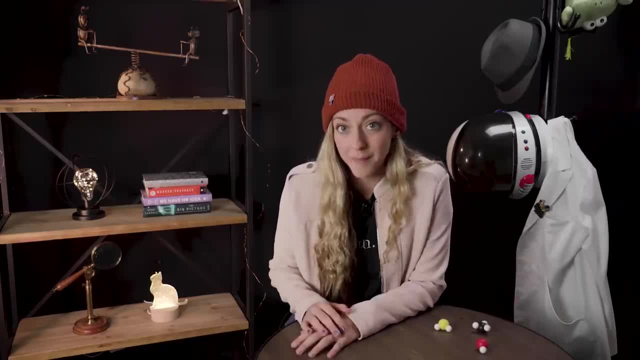 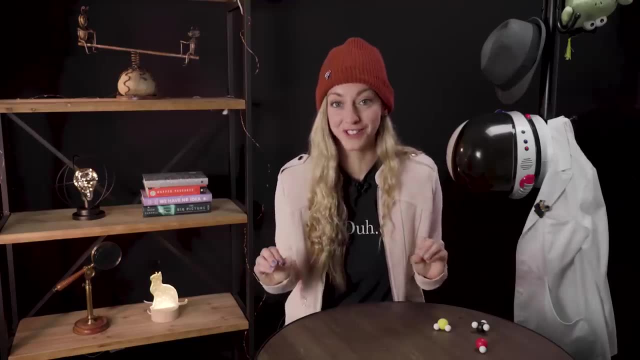 the electron field, Just like if there's no hill on the topographical map, there's still a number value to represent the elevation there. Particles are like little hills in the quantum fields. They're actually vibrations. They're vibrations in the field, which kind of starts to make it clear on how a particle 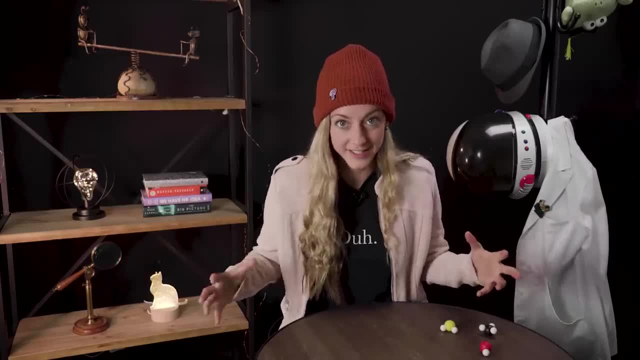 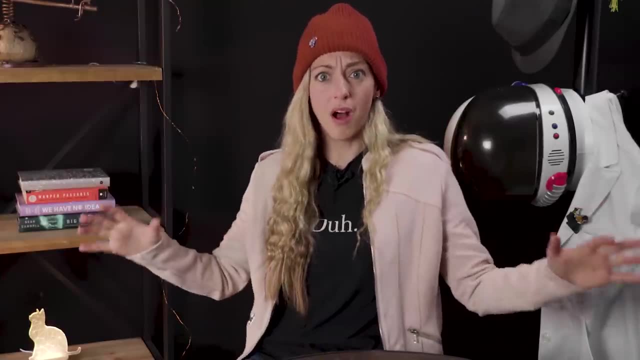 can act like a wave. The quantum field exists even if there's no particle in it, just like an ocean can exist even if there's no wave in it. This seems like a good moment to pause for dramatic effect, because all the stuff that 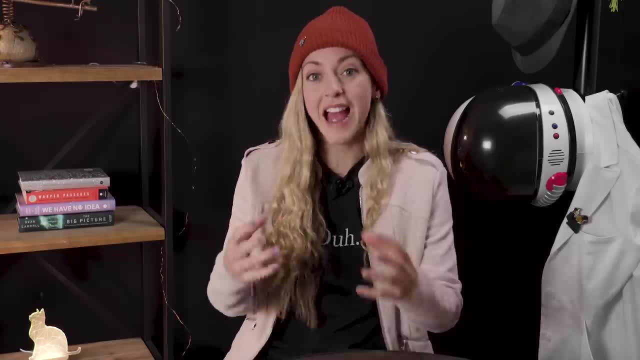 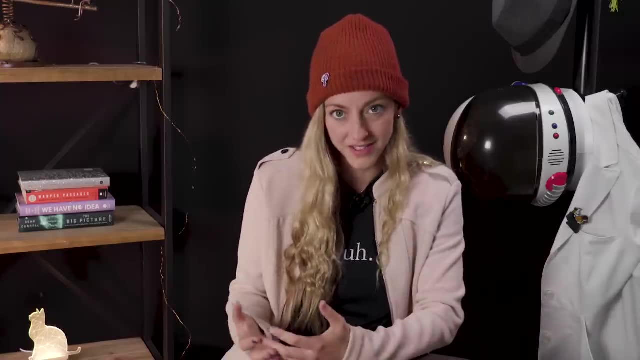 we're familiar with. that we typically describe as being made of particles is actually made of a bunch of fields. I'm not even going to say so cool, because I can't even wrap my head around this. This is so bizarre. 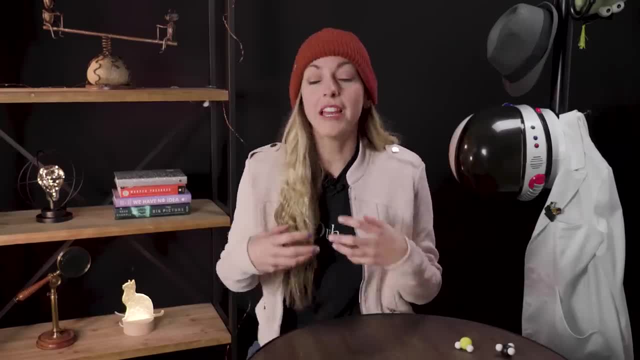 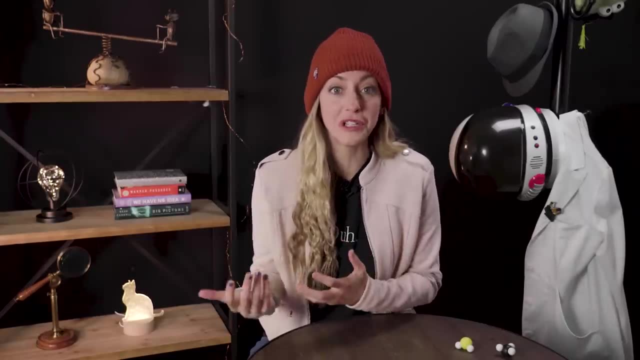 More bizarre is that particles are not absolute. Particles can appear to exist for one person looking at the field and not for another, depending on how fast they're both moving, which has to do with changing reference frames. The particle that can travel at the speed of light will travel at the speed of light. 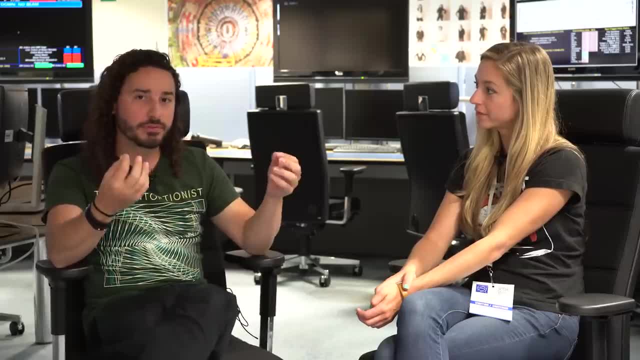 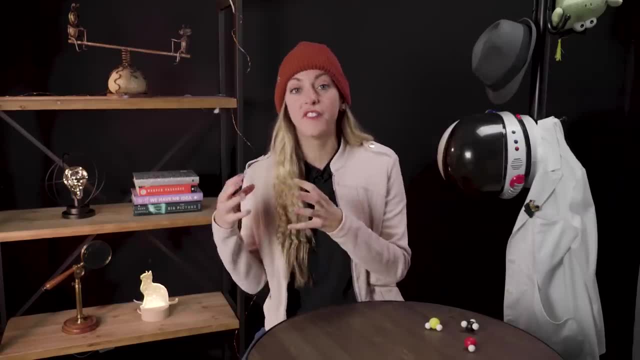 The fact that you're traveling slower than the speed of light means that an observer, a different observer, you can change reference frames. If you're moving super fast, like close to the speed of light, then the value of the clock changes, which is kind of like time dilation, the phenomenon where, if you're 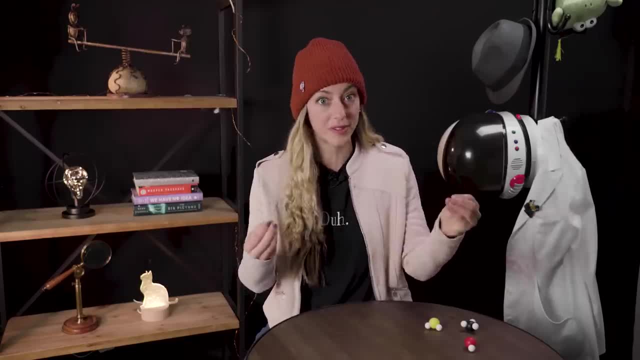 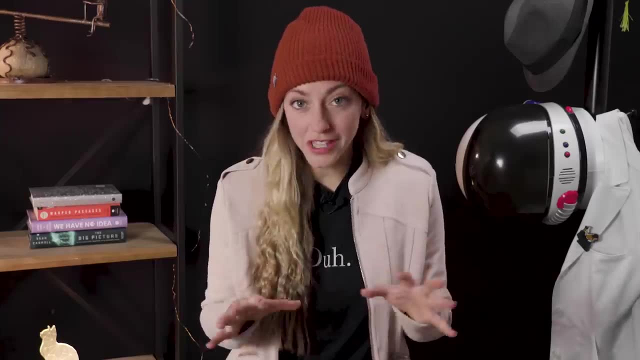 moving fast, then your clock appears to tick slower than a person who's stationary, Which is a real thing that if you've never heard of, then I envy how blown your mind is right now. So this all indicates that the fields are fundamental and not the particles. 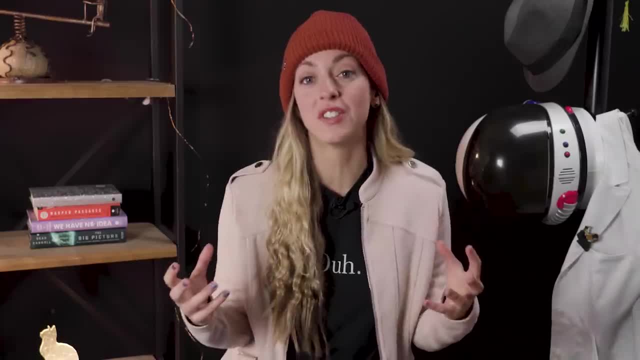 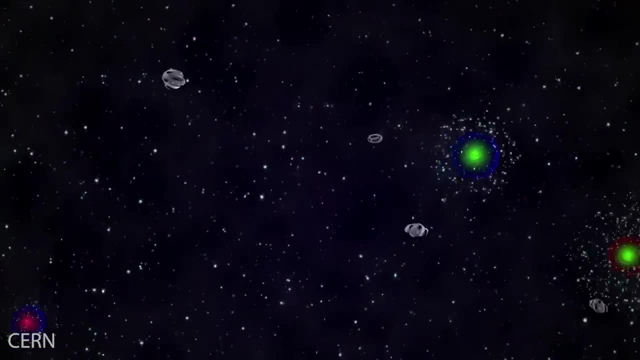 And once you start to think in terms of the fields, then the experiments at the LHC start to make a lot more sense, Because the LHC smashes protons which are made of two up quarks and one down quark, held together with gluons. 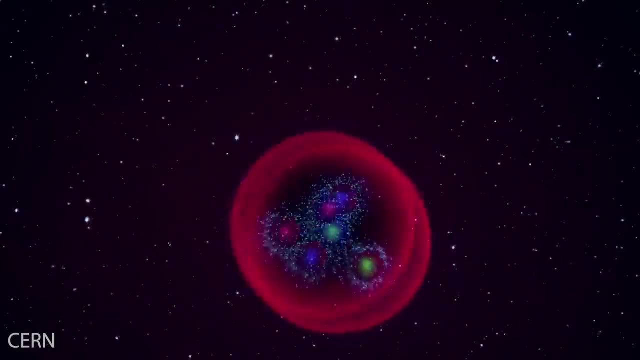 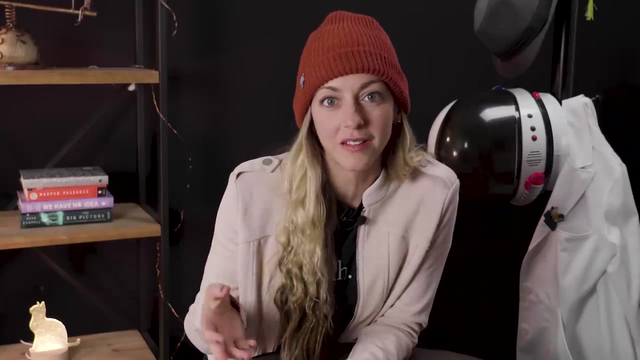 So you might have thought that you get a mess of quarks and gluons out of the collision, like I initially thought, But they managed to get Higgs boson. It's like you blended up a bunch of fruit in a smoothie and popped out a chicken nugget. 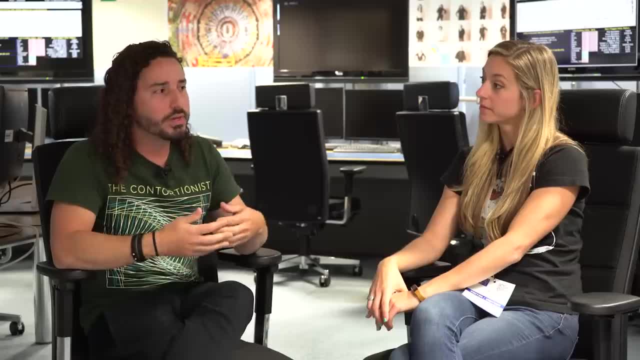 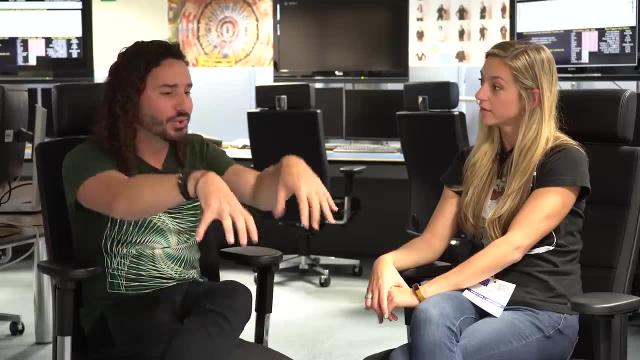 But the thing is, the quantum fields can interact. One way you can see it is: there's this sort of instrument or musical instrument analogy, where you might have maybe a piano strikes a chord And if there's other instruments around, there might be resonance, right. 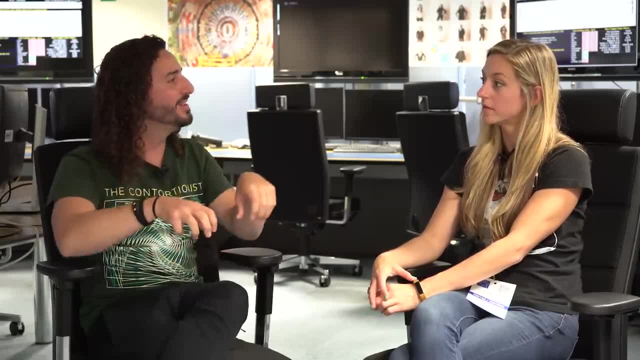 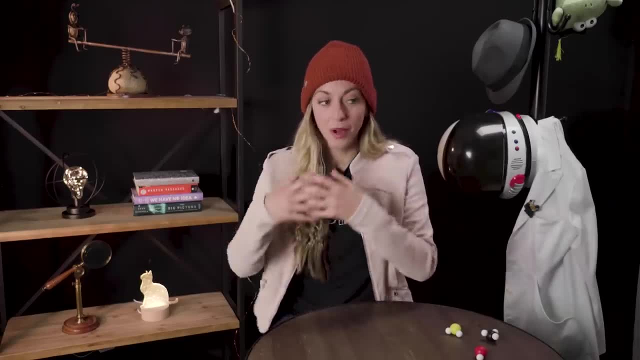 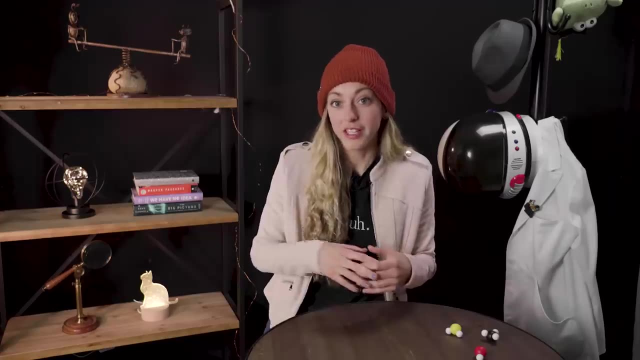 So one of the strings on a guitar might start vibrating because the piano is hitting the right note. So it makes more sense if you think that collisions are creating great disturbances in the quantum fields. rather than thinking about particles colliding, You can imagine the energy of one field transferring to another and another like a vibration in. 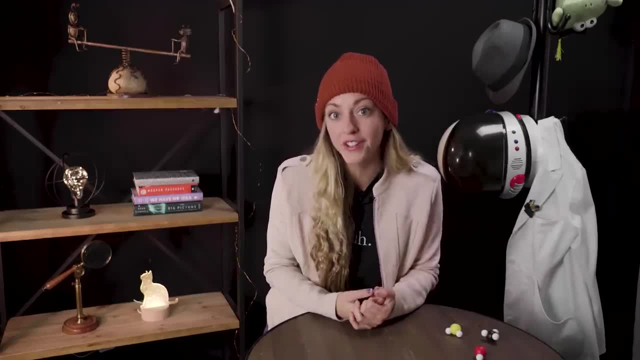 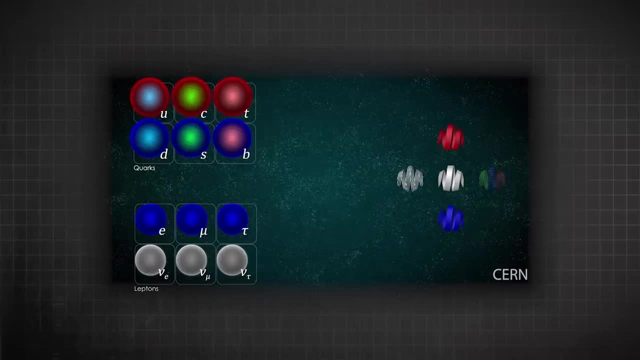 the up quark field, causing a vibration in the electron neutrino field or the Higgs field. Speaking of the Higgs boson, which was the most elusive particle for physicists to detect in the standard model of particle physics… I'm not really going to go into the significance of it or what it is, because there's so much. 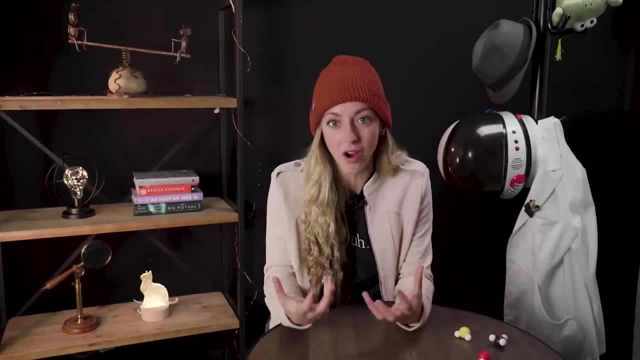 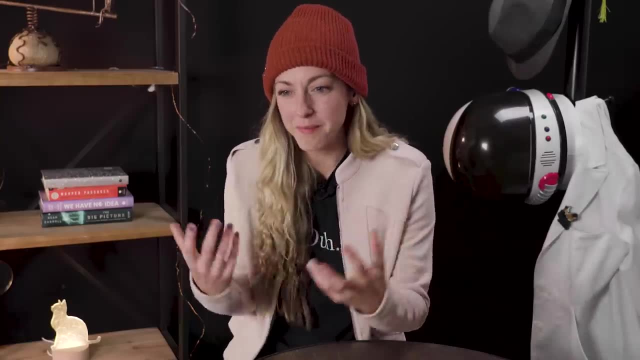 material out there on the internet about it. But now that we understand what particles are, I want to talk about how we detect the Higgs boson, the insane sensitivity of detecting it and the crazy methods, Because we don't actually ever directly detect the Higgs boson with detectors like 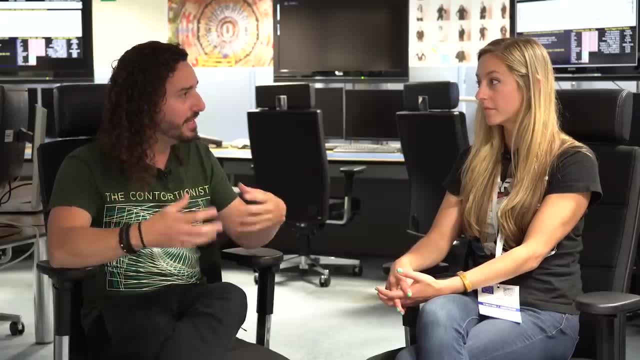 CMS. So how do we do it? The decay products from the Higgs decay are fundamentally indistinguishable from the decay of other particles. Decay products refers to the fact that particles like the Higgs boson are fundamentally indistinguishable from the decay of other particles. 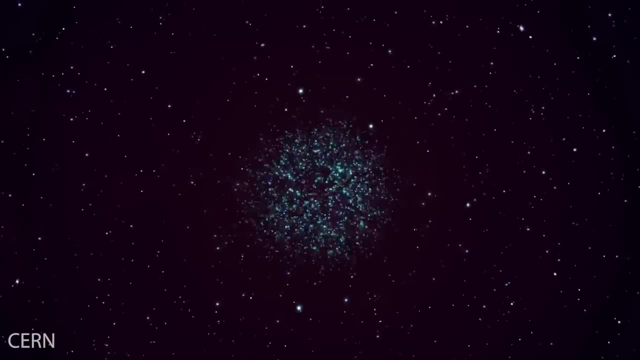 Decay products refers to the fact that particles like the Higgs boson are fundamentally indistinguishable from the decay of other particles. Decay products refers to the fact that particles like the Higgs boson are fundamentally indistinguishable from the decay of other particles. 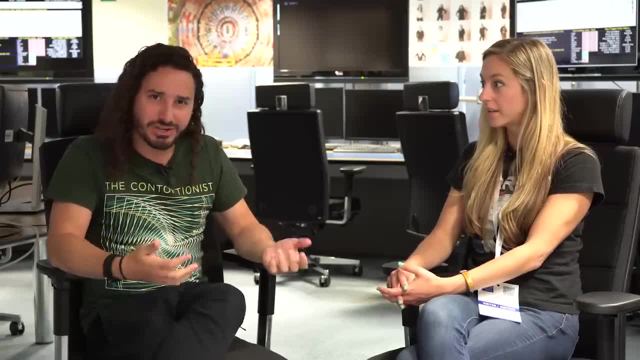 Decay products refers to the fact that particles like the Higgs, which are unstable, can spontaneously turn into other particles. So a scientist that's trying to find a new species that's invisible, well, what you do? you have to look at the decay products. 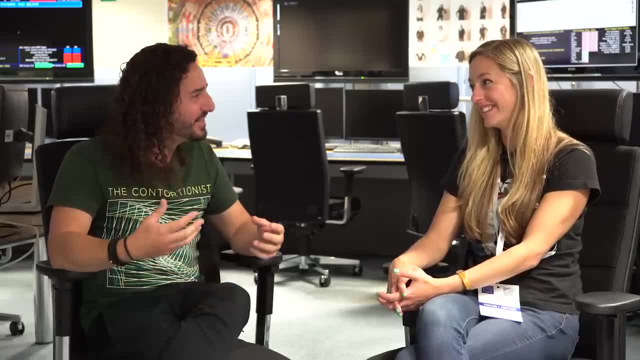 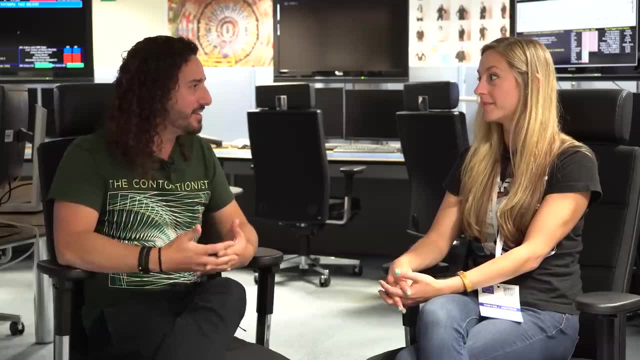 So let's look for poop, right. And then, how do you distinguish this animal, this new species, poop, from other species? The answer is that you don't. You can't. If you produce a Higgs particle, again, you don't see the Higgs, you have a bunch of poop. 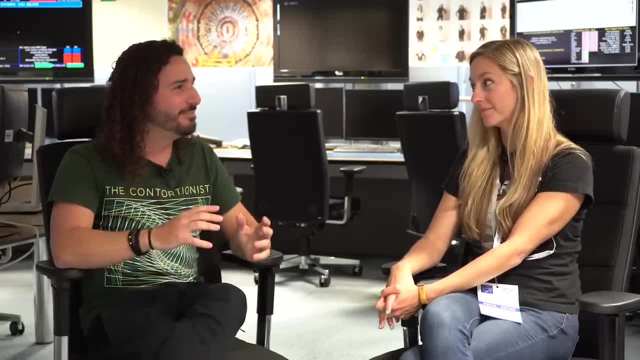 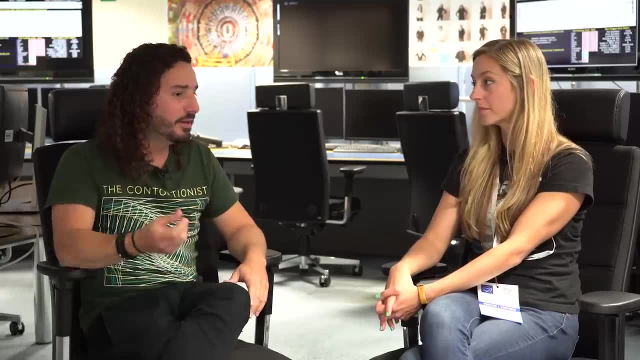 in the forest. That's the challenge is, you have to be super confident in your prediction And then you have your measurement. You have to go to the forest and actually find this poop. What if you think this is poop, but it's, I don't know, mud, I don't know, no idea. 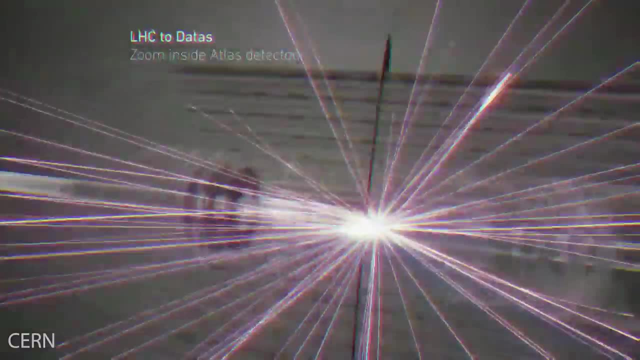 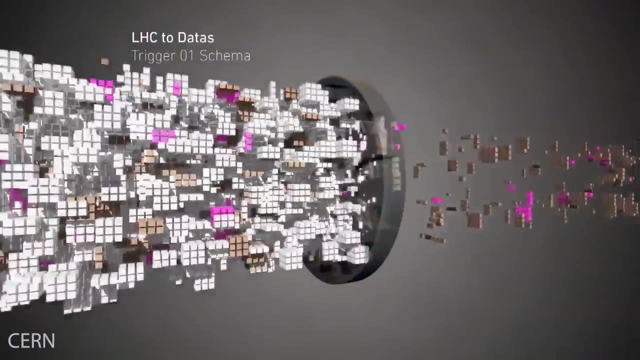 Can you? is there anything in the poop that you can use to identify the species? You can see why we need a lot of data. You only produce the Higgs very rarely in these collisions. Another way to say this is that most of the poop that you think comes from the Higgs comes 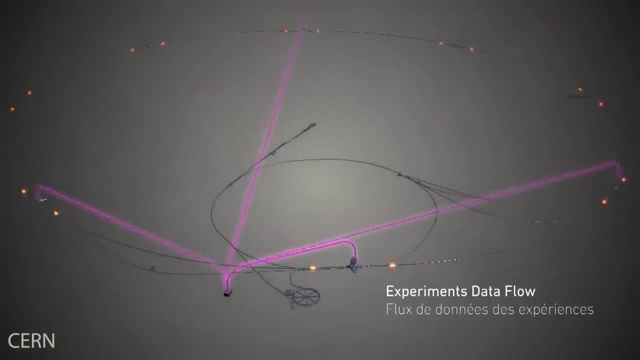 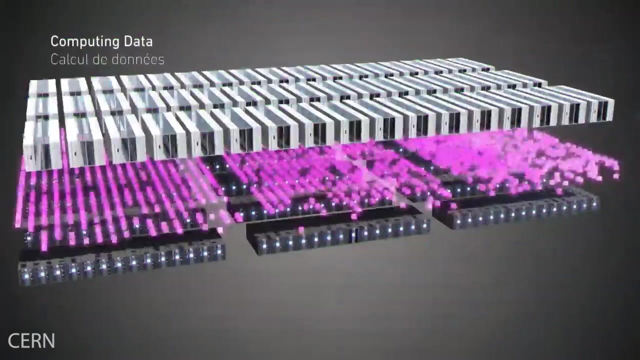 from other species. You have to be very confident about your data, About your prediction, And be very confident about your measurement. If your prediction and your measurement match exactly, Let's say you somehow calculate, okay, we're going to find 100,000 poops. 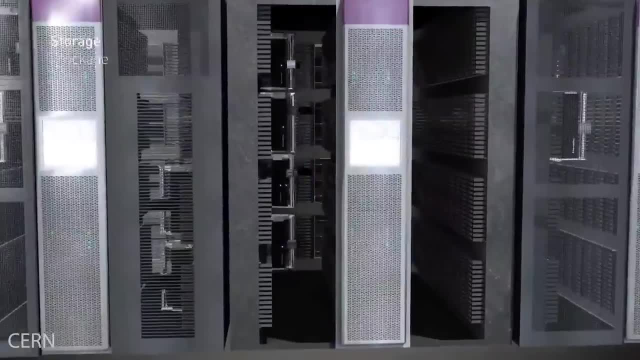 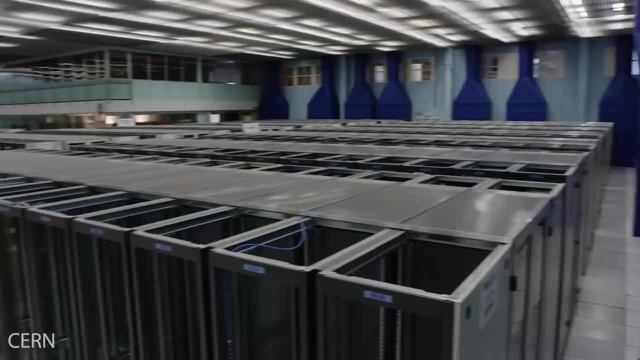 And you find 100,200.. There's an excess of 200.. Is that significant? So that's why, when we discovered the Higgs, we had to have a lot of data And that's why it took so long. We needed to compare the prediction to the observation. 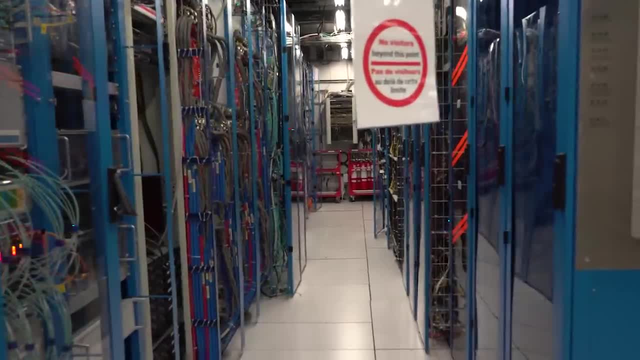 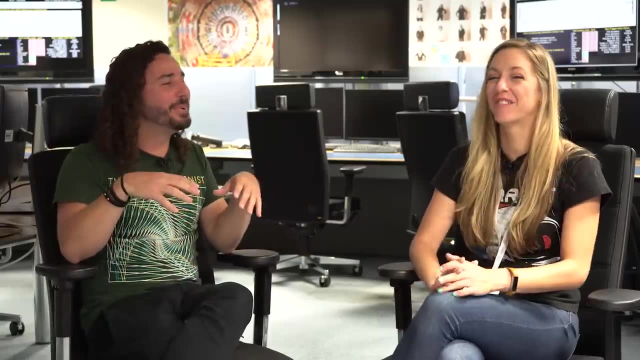 And when we finally said we did discover the Higgs, it was actually after we had many, many collisions. Sorry if this analogy is kind of gross, by the way, but I was pretty happy with the fact that you used poop. That was my first thought. 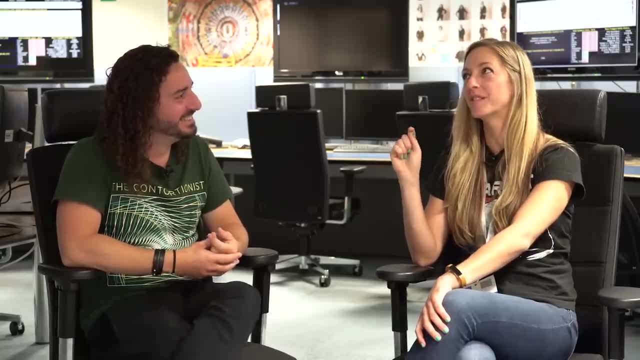 I was like: oh, you could use poop. And I was like I shouldn't say that You could also use footprints. And then you said poop And I was like, yes, Well, yeah, I usually use footprints for this analogy, but Sarah encouraged me to go for. 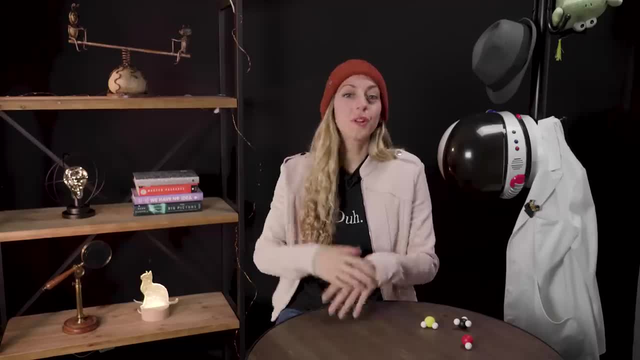 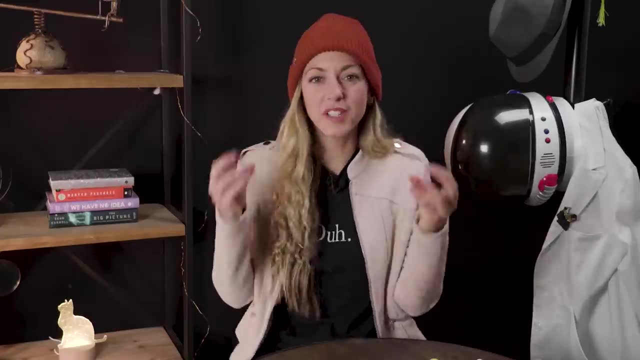 poop, Go for the poop, Go for the poop. So we're looking for an excess of poop. It all makes sense now, Except, why do we need all of that, The giant colliders, the massive detectors? why do we have to smash protons at such high? 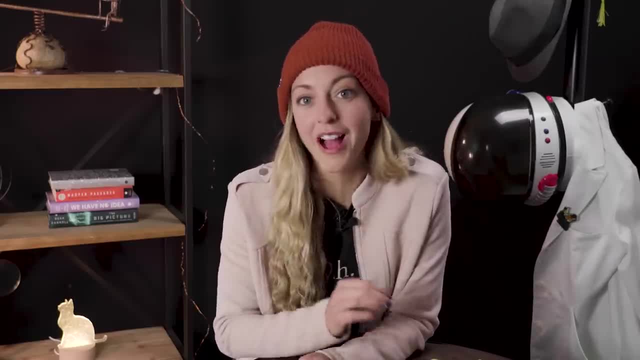 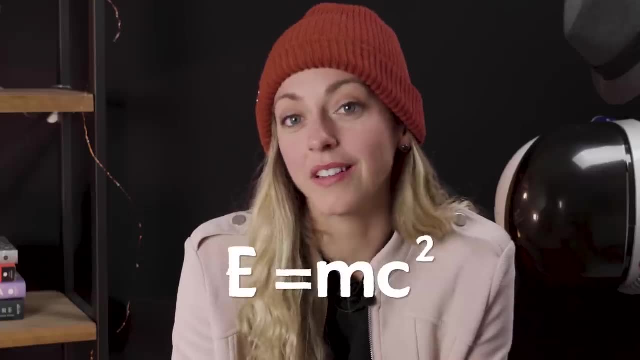 energies. Well, the Higgs boson is the second heaviest fundamental particle after the top quark, And the heavier the particle, the more energy you need to produce it. E equals mc squared, Thanks Einstein. So if you transfer enough energy into the Higgs field, you get a Higgs boson. 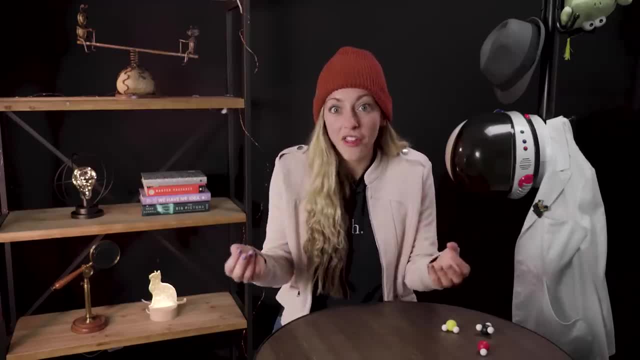 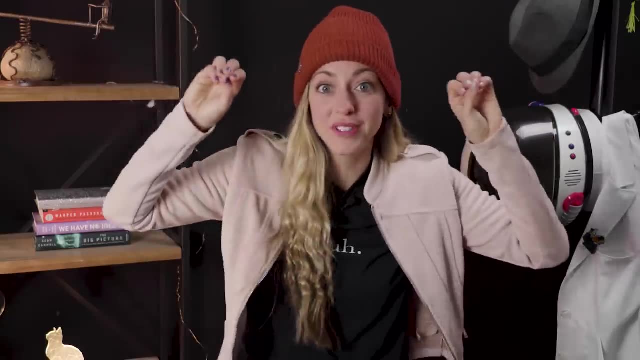 So you need a lot of energy to make particles out of seemingly nothing. But then you need massive detectors to see all of the data, All of the debris that comes out And all of the particles that those particles decay into, because there's a ton of it. 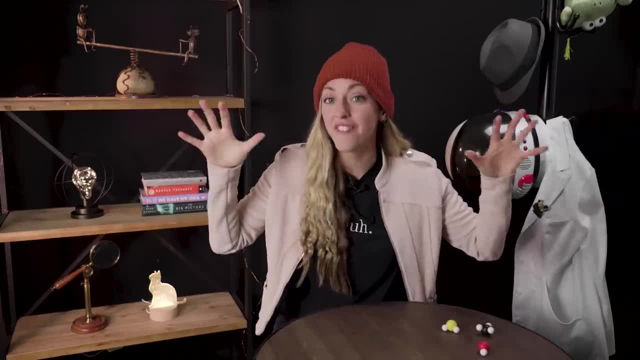 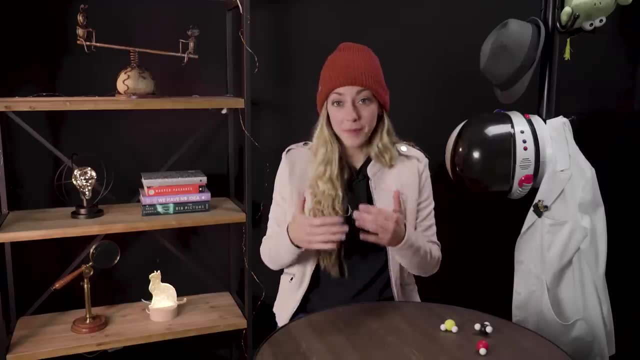 And they're all going really close to the speed of light, So they're going to make it pretty far, pretty fast. So you need massive detectors with massive magnets and massive numbers of wires. But let's rewind a bit, because the whole purpose of making this video is that I went. 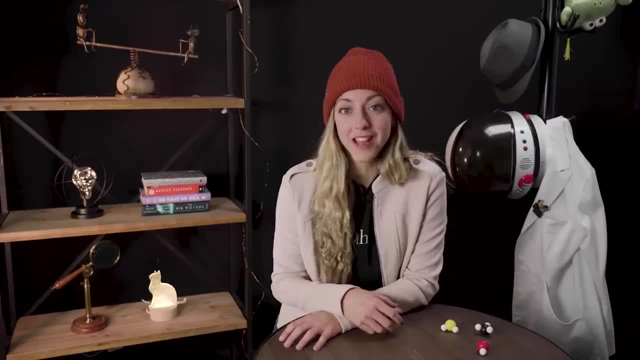 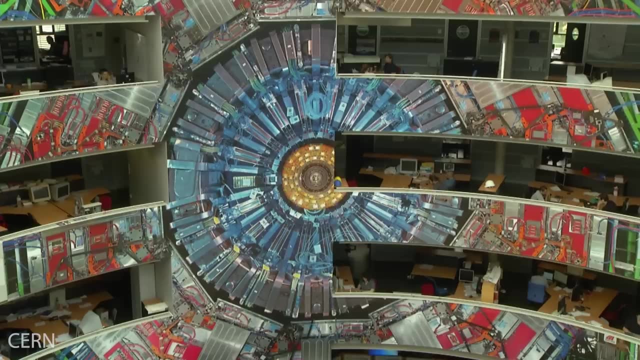 there. I went to see these detectors So I really wanted to know what it was like to work with them. What's it like to work at CERN? It's a little bit like a college campus. Yeah, It's complicated. It's sort of like everybody is on that mission. 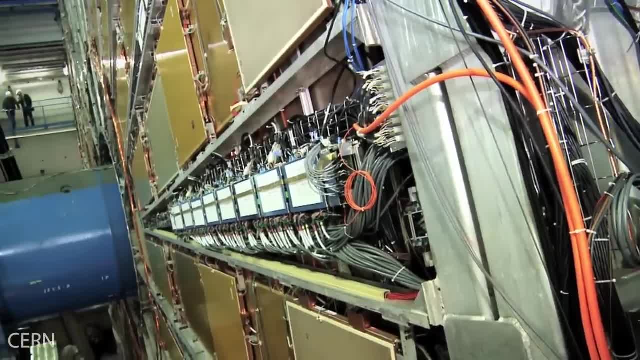 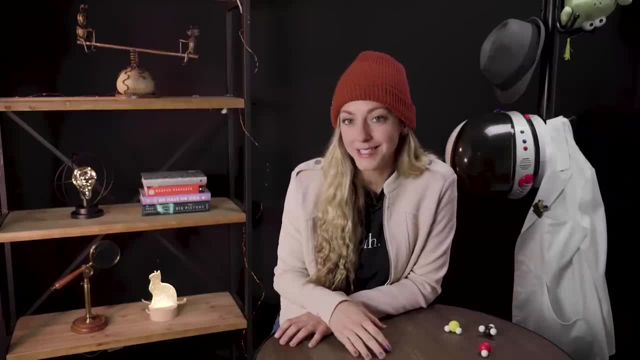 Let's try to understand the universe. People here are super passionate. I feel, like people here would be willing to work almost for free, That their motivation is to understand the universe. I very much support scientists getting paid for the amazing work that they do. 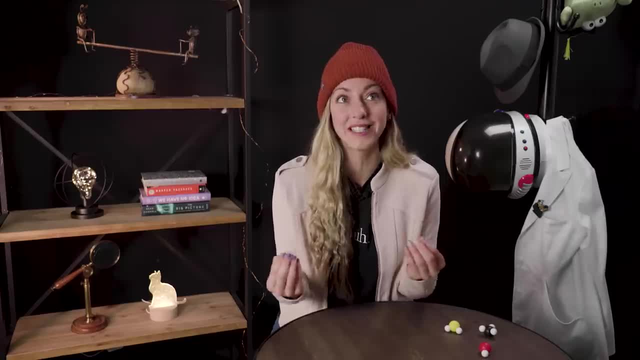 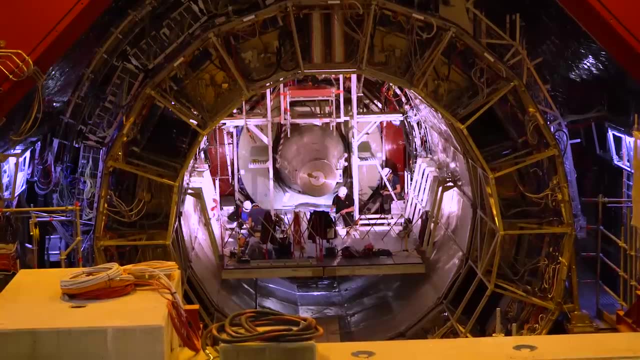 But I definitely understand the excited sentiment because it was almost as exciting being there just visiting. So were they colliding particles while we were there? No, See those guys. They were in the beam path. No one is in the beam path. 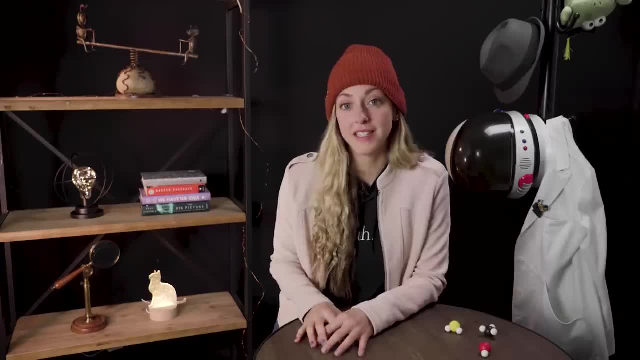 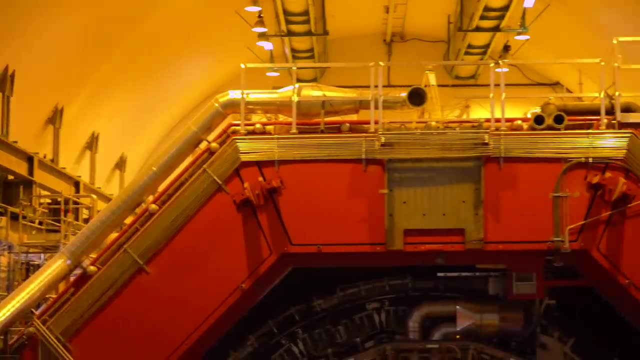 No one is in the beam path when it's on. CERN has been in shutdown since December 2018, and it's going to reopen in 2021.. Then they'll close those giant magnetic doors we were looking at and it'll take an entire 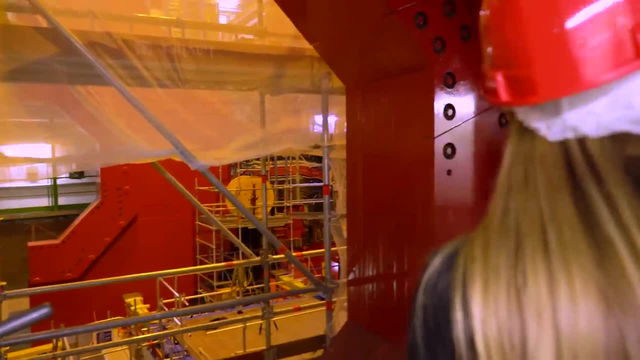 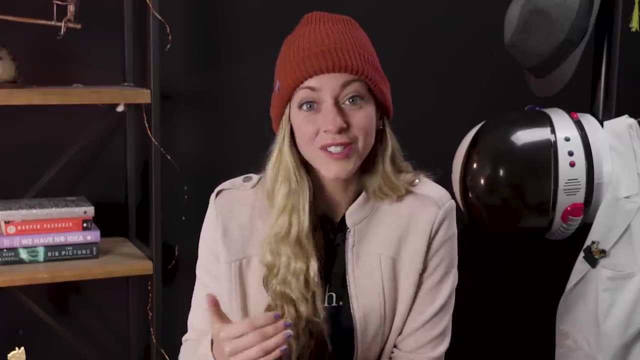 day to do so, because they weigh hundreds of tons And you don't want to bump a multimillion dollar magnet. But it was super lucky that it was shut down when we went, because we got to go underground and see everything. There were wires everywhere. 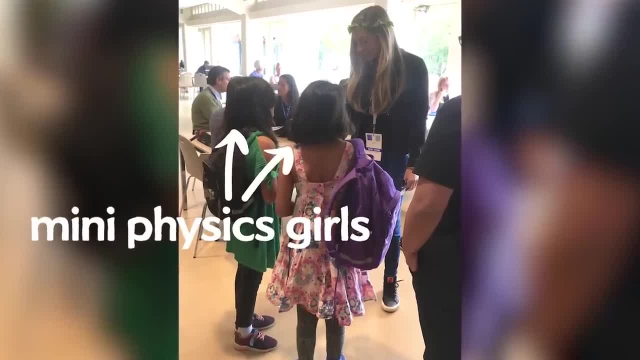 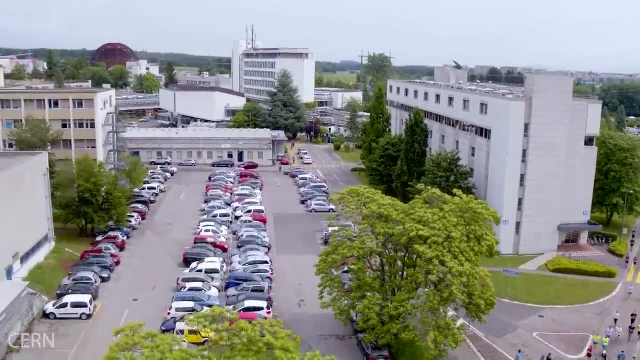 Cables and wires are like the wallpaper of CERN, And the internationalness was so noticeable. Every person that we met was from a different country. So the US is a very large collaboration, over 3,000 people. So what's next for particle physics at CERN? 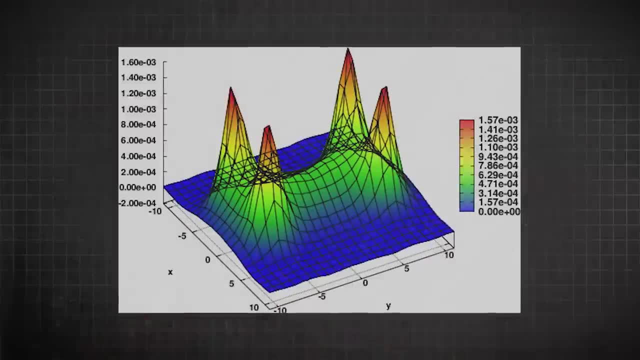 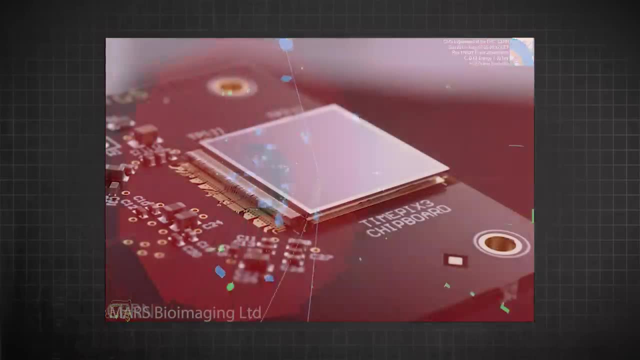 Well, just in 2018, they made some crazy discoveries, like finding evidence of another exotic particle made of four quarks, a terra quark- Precisely measuring the spectrum of anti-hydrogen, And making the first 3D color X-ray of a human body which is based on technology developed. 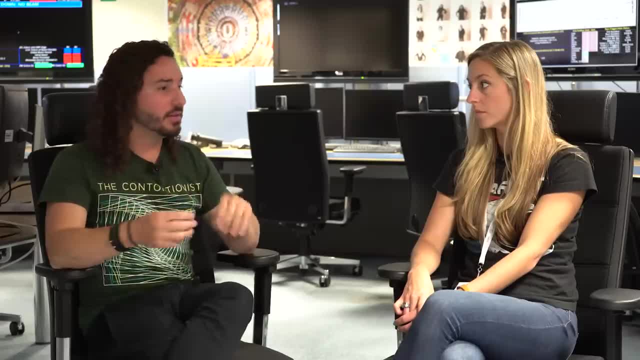 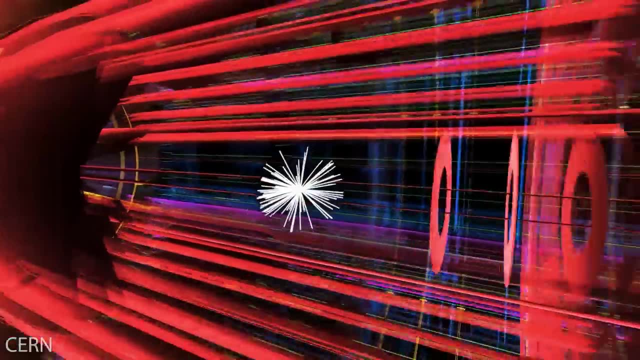 at CERN And in the future, hopefully, dark matter- Maybe not dark matter, but maybe we find some other type of particle- decays into dark matter and this other type of particle. maybe it lives pretty long like, maybe it lives for a while. 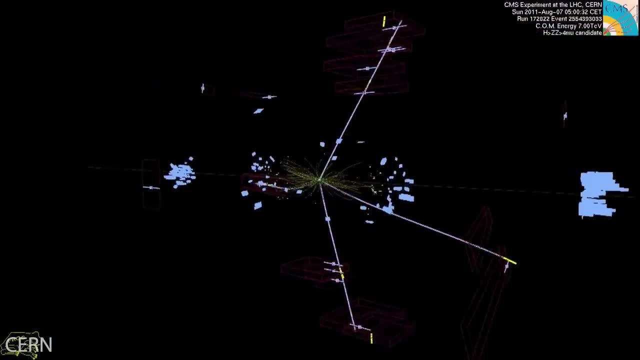 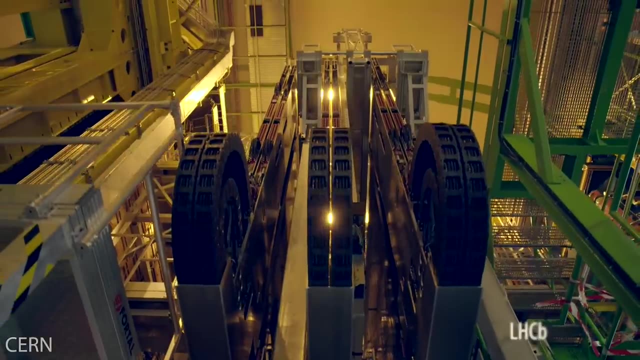 So that means they can have a collision and then a particle pops out, Maybe it moves outside your detector and then it decays into dark matter. So you're missing that. We have our detector 100 meters underground. We're considering to install detector modules in the surface in case one of the particles 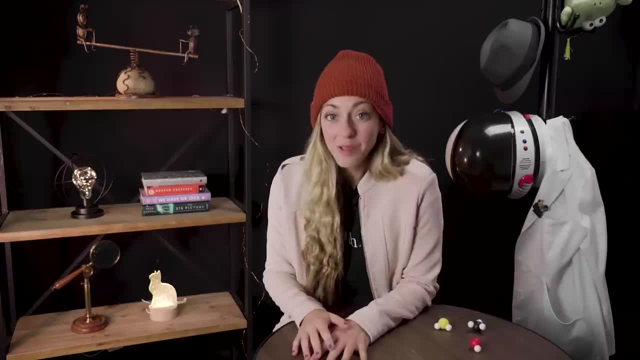 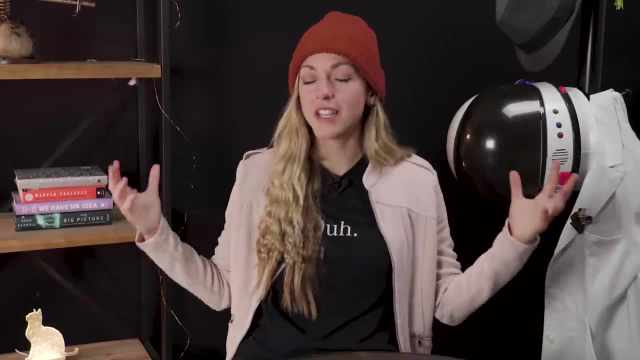 travels 100 meters to the surface and then it decays. I'm super pumped to see what happens when CERN turns back on in 2021, because that collaboration of thousands of scientists and engineers from around the world are digging into the fundamental physics of our universe. 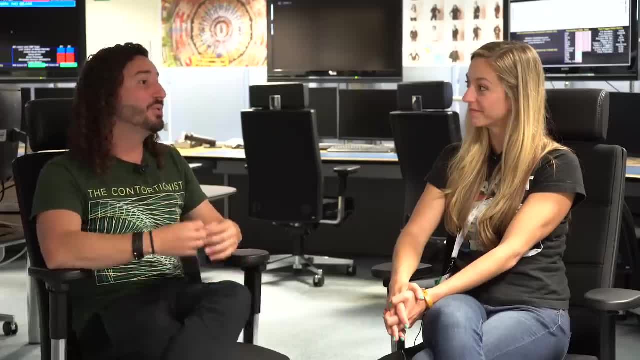 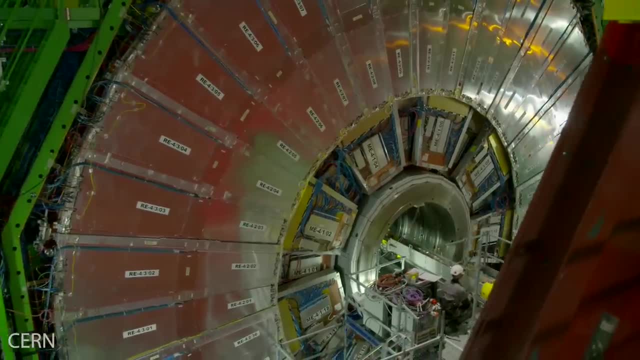 And that is cool. It's hard for me to understand how we would not be fascinated at what we do here. It's really remarkable, And the fact that this all works as well. like I mentioned, all these careful predictions, this careful measurements.